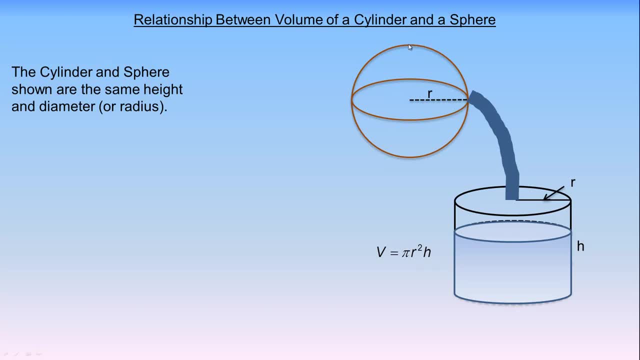 And you see, this height here is actually two radiuses, because that would be a radius and then that would be another radius and this is supposed to be the same height as this cylinder. So the height is actually two radiuses, or h equals 2r. 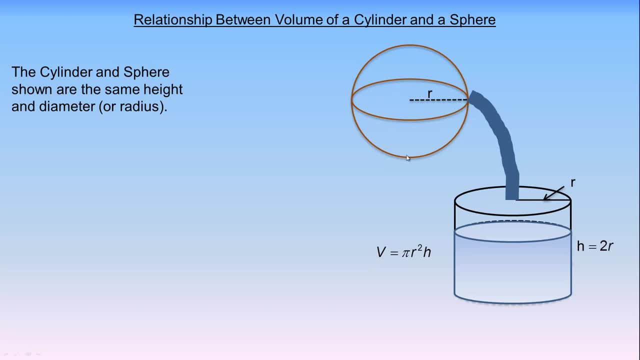 So I can find a formula for the volume of the sphere by multiplying this by two-thirds, because this whole thing, it's two-thirds of the cylinder, So the volume of the sphere. and this isn't a usable formula right now, but it will be in a moment. 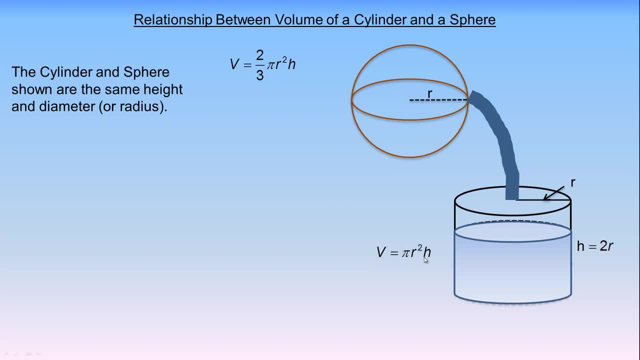 So it's two-thirds times this pi, r squared volume formula for the cylinder. So what I'm going to do is there's no height in this. I'm going to replace the h with 2r, because that's what the height of this would be. 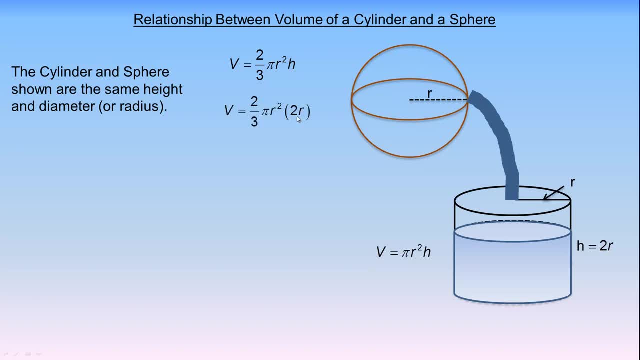 It would be two of these r's, So I'm going to put a 2r in place of the h. Everything else is the same. two-thirds here, pi, here, r squared here, And I'm going to kind of break this 2r up into. I'm going to multiply the 2 by the two-thirds. 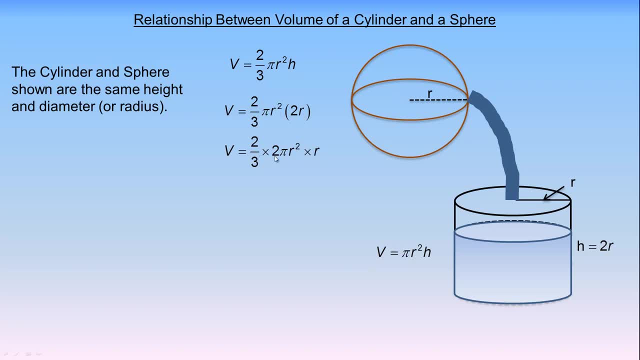 and of course, the r is going to get multiplied by the r squared here, Now two-thirds times 2, how do you do that? Okay, this 2 is the same as having a denominator of 1, same as 2 over 1.. 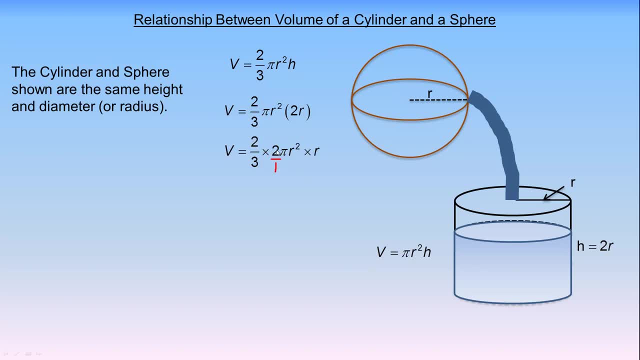 So when you multiply this 2, you multiply the two 2's in the numerators. That's going to be 4 over 3,. 3 times 1 is 3.. And then r squared times 2. 3 times r, remember, you add the exponents. there's a 1 here and a 2 here. 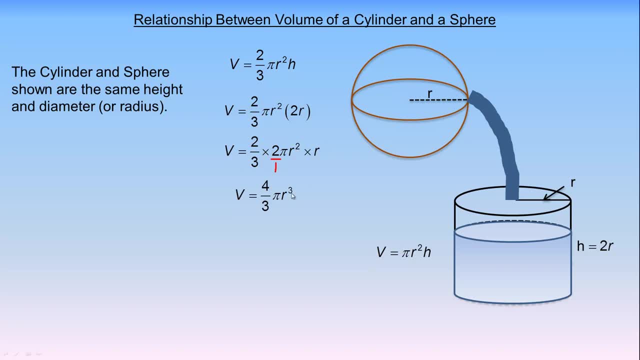 So there's actually two r's here and another one here, so there's three all together. So the volume formula for the sphere is four-thirds pi r cubed, And that actually is the volume formula for a sphere. It's four-thirds pi times the radius cubed. 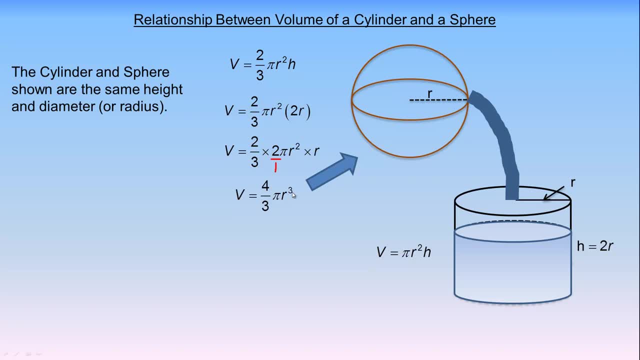 So that just shows a relationship between the volume of a sphere and a cylinder and how you actually can derive the the volume formula for a sphere from a cylinder. And that's the end of the tutorial.